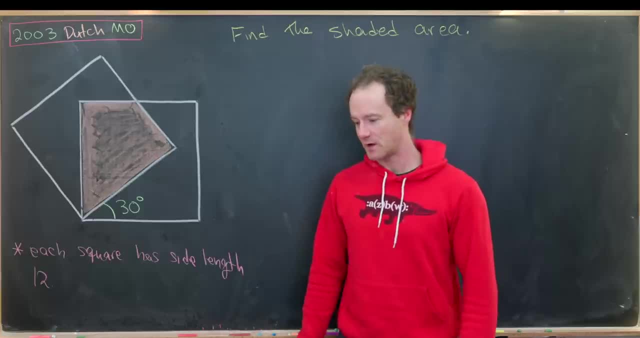 that we're talking about it. maybe, if you guys want to post in the comments what you think, maybe the most ridiculous way to do this problem is, before I go into the solution and see if you guess, right. Okay, so let's look at the problem. What we have here are: 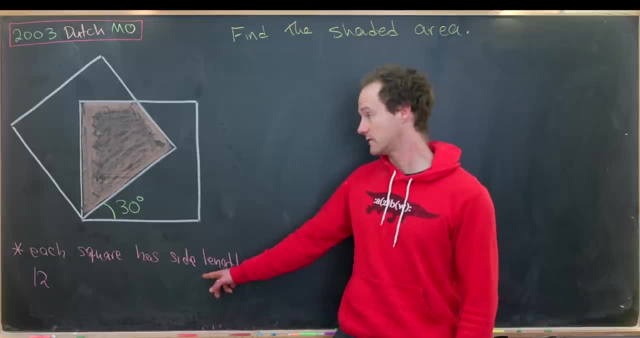 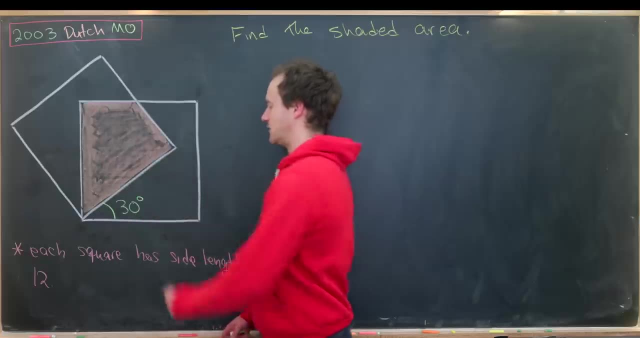 two squares of side length 12. So they share a vertex over here. And then this one that's rotated has been rotated 30 degrees And our goal is to find the shaded area. So that's this area right here which is contained in each of these squares. 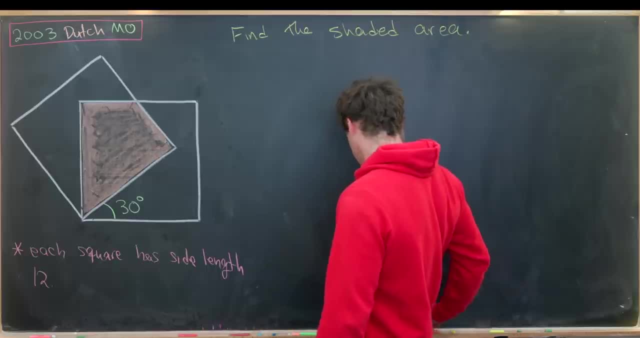 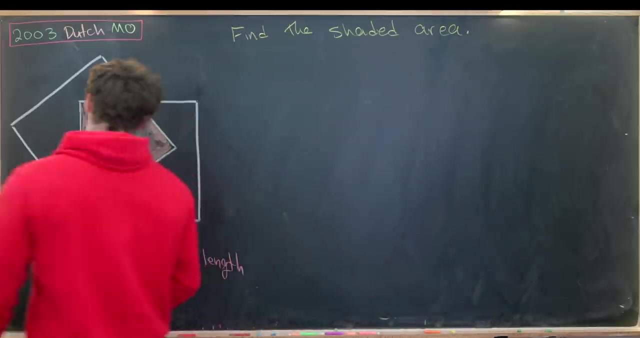 Okay. So, like I said, now is your chance to think about the ridiculous way that I'm going to solve this and what that says about me, and post it in the comments And we'll get going. Okay, so what I'm going to do is put this in the Cartesian coordinate plane. So this: 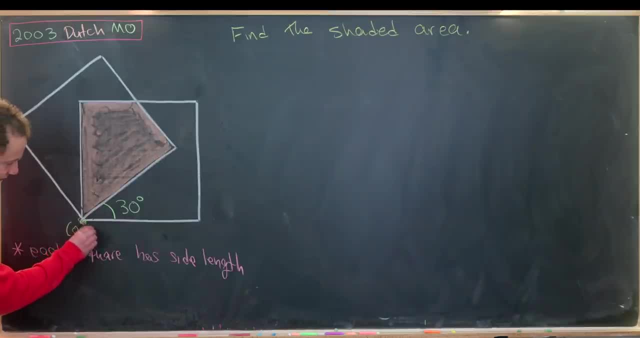 point right here. I will make the origin. So this is the point: zero, zero. And then this is along the x axis, making this point right here: 12, zero. This point up here is 12, zero, And then this point over here is 0, 12.. Now we're going to start filling in the rest of. 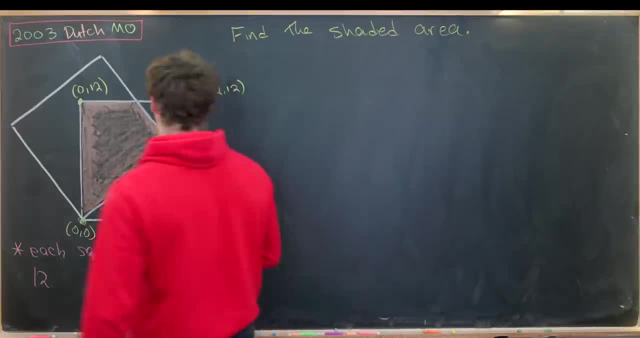 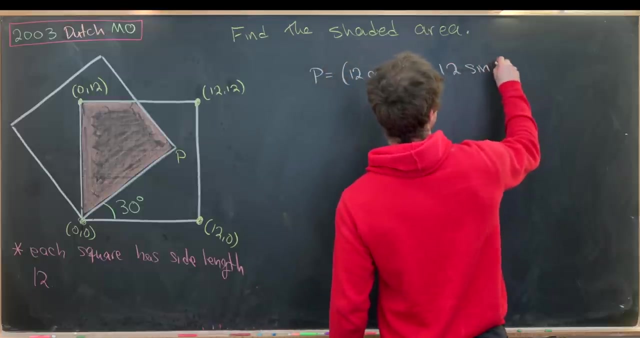 this stuff. So notice this point right here. maybe for now I'll call it P- will be of the following form: So P is going to be equal to 12 times the cosine of 30 degrees, and then 12 times the sine of 30 degrees, And we can see that just by looking at the graph. 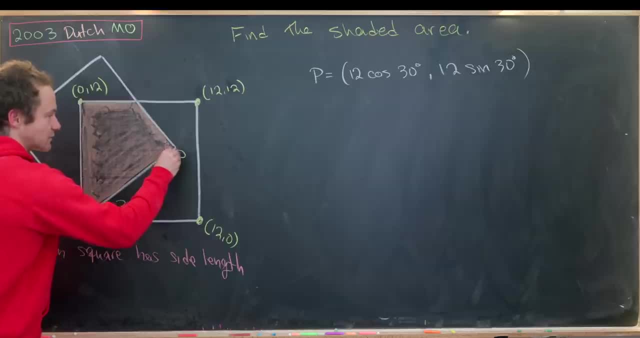 Okay, so this is the cosine of 30 degrees And then 12 times the sine of 30 degrees, And we can see that just by looking at the graph. So this is the cosine of 30 degrees And we can see that just by completing this right triangle right here. So if we complete, 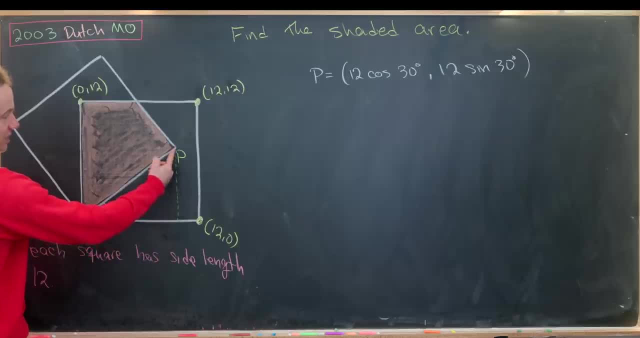 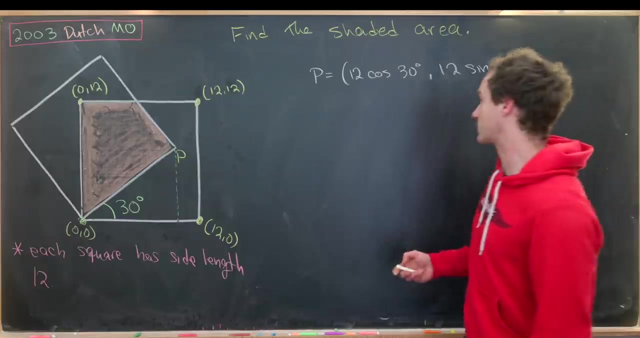 this right triangle, we'll notice that the height of the right triangle will be the y coordinate of P, whereas the base of the right triangle will be the x coordinate of P. Okay, so now we'll use the fact that the cosine of 30 degrees is the square root of 3 over. 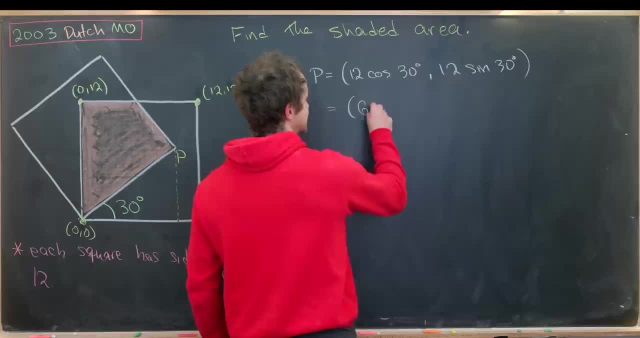 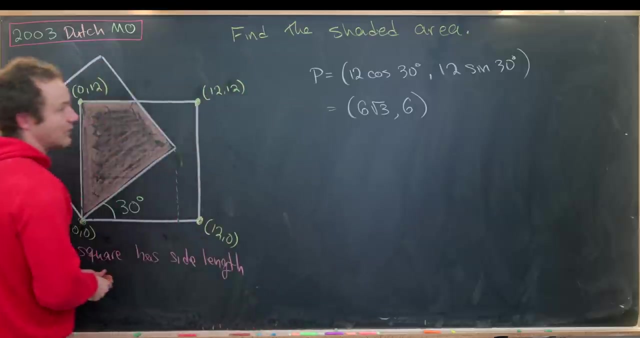 2 to rewrite the x coordinate as 6 times the square root of 3.. And then the sine of 30, 30 degrees is a half, so that gives us 6 for this y-coordinate. Okay, so now that we've got that, we can erase this p and then write down the coordinate for p that we just calculated. 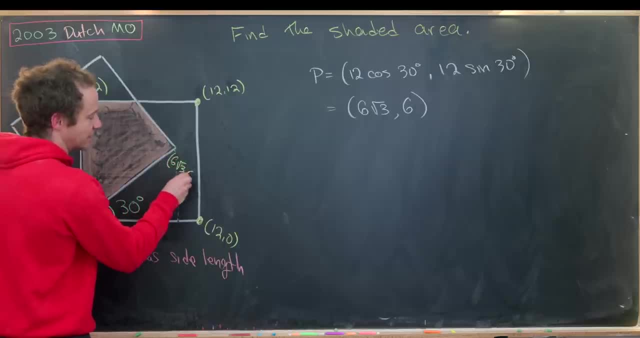 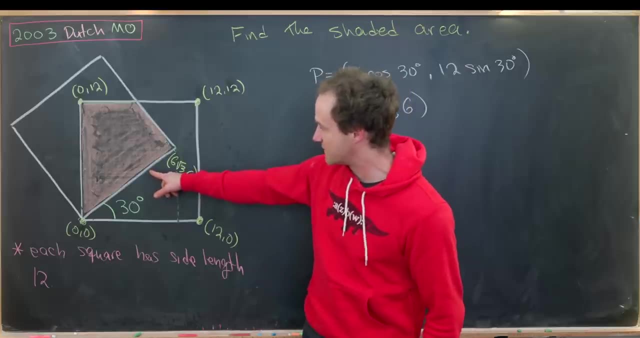 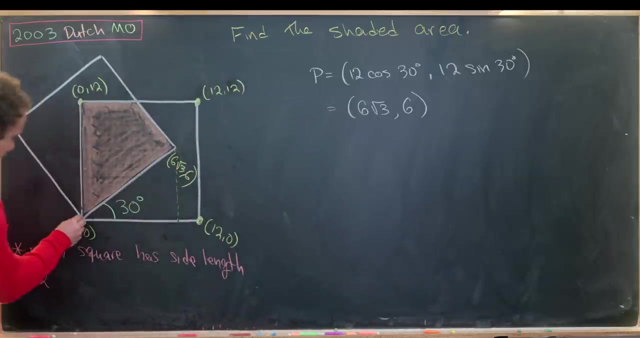 So this is 6 times the square root of 3 comma 6.. Okay, great. Now what I want to do is write the equation of this line right here, And so really it's just a line segment, but you could think about it being extended to a line and it will have an equation. 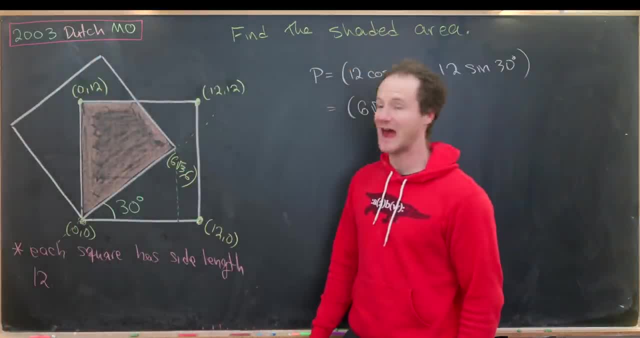 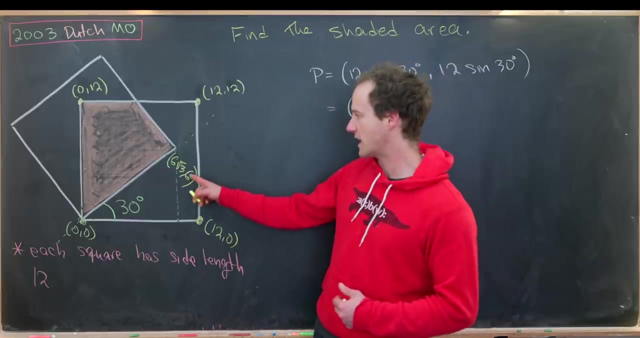 Or you could just think about it as a line segment where you restrict the x value inside of the equation of the line. But notice that the equation of this line is very easy to calculate, And that's because it goes through the origin. So all we need is the slope. but the slope will just be the y-coordinate here divided by the x-coordinate here. 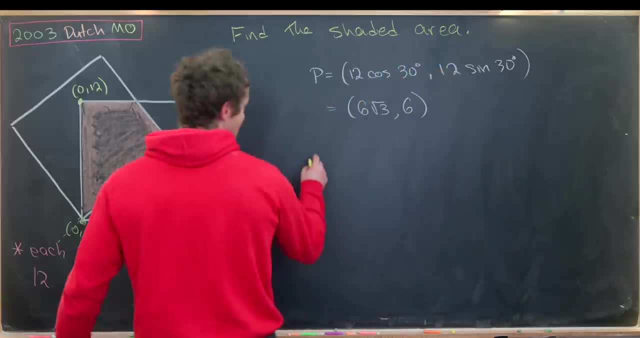 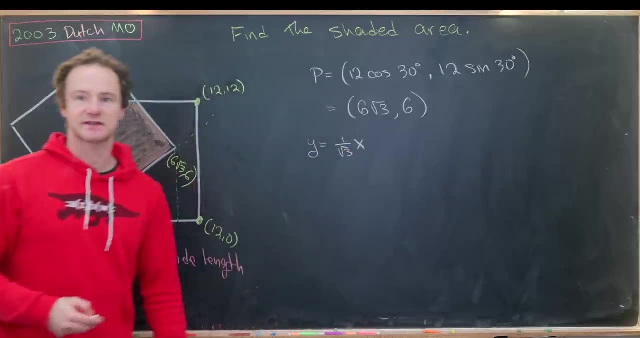 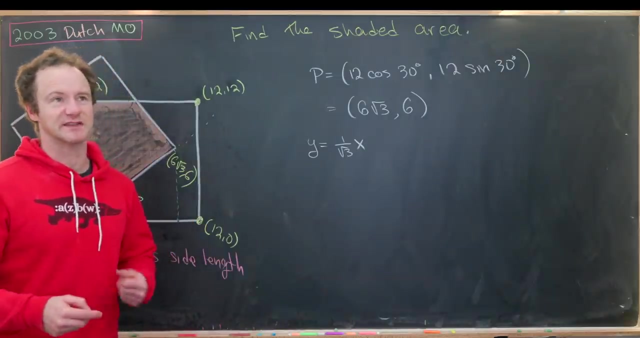 So notice that. Notice. this line has equation- Maybe I'll write it over here- of y equals 1 over the square root of 3 times x. Now, generally I don't rationalize the denominator, but I'm going to do it in this case because it will let this term interact with some that we'll see a bit later. 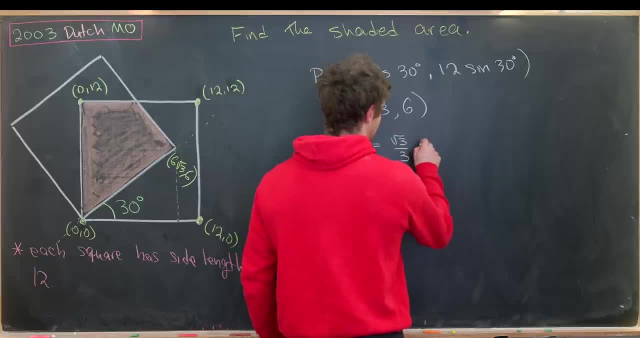 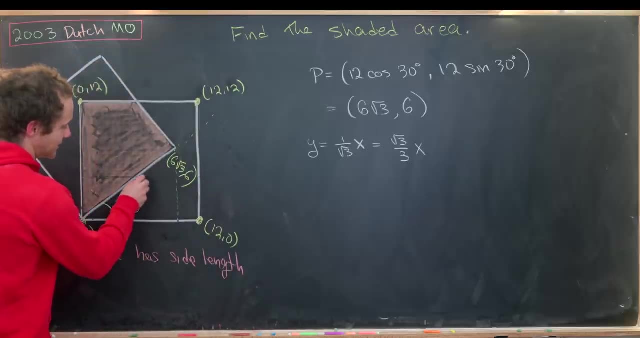 So this is the same thing as the square root of 3 over 3 times x, Just like I said by rationalizing the denominator. So let's put that In here, right here, so I don't want to make it too messy here. 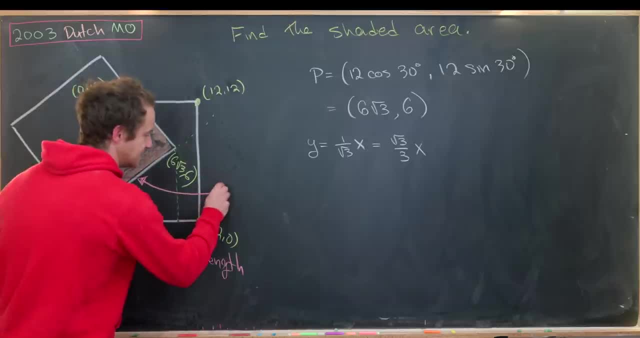 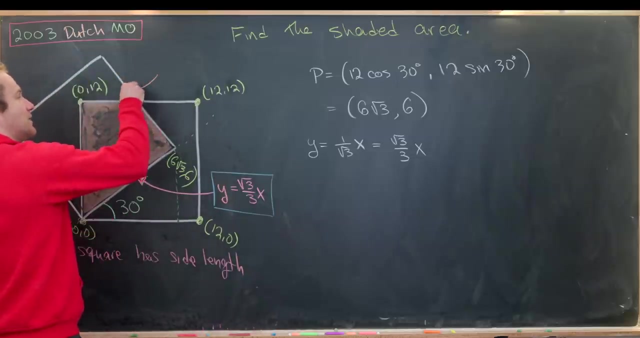 We'll note that this line right here has the equation: y equals square root of 3 over 3 times x. Okay, that's good. Now next up, I want to find the equation of this line up here so we can use the fact that this is a right angle. 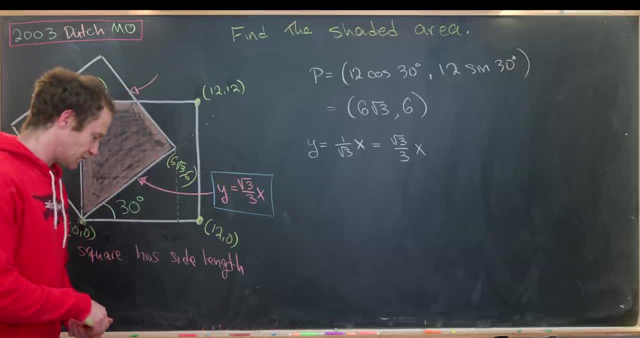 So these two lines are orthogonal, So let's put that In for now. We know the slope of this line immediately. So the slope of this line will be the negative reciprocal of the slope of this line. But we might as well use this version, the slope of 1 over the square root of 3, because taking the reciprocal is a little bit nicer there. 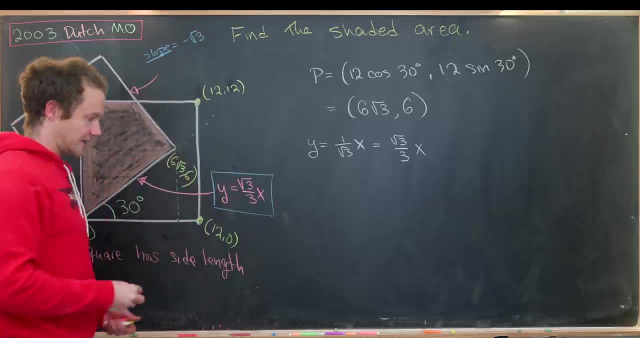 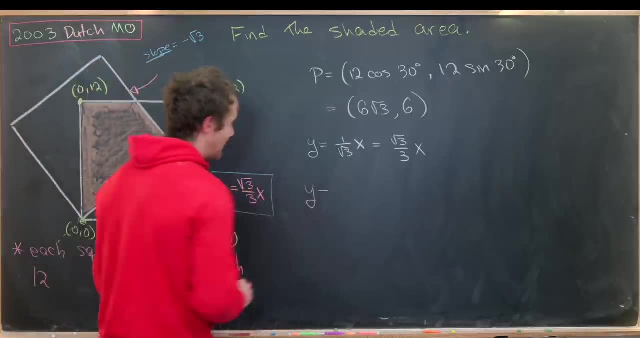 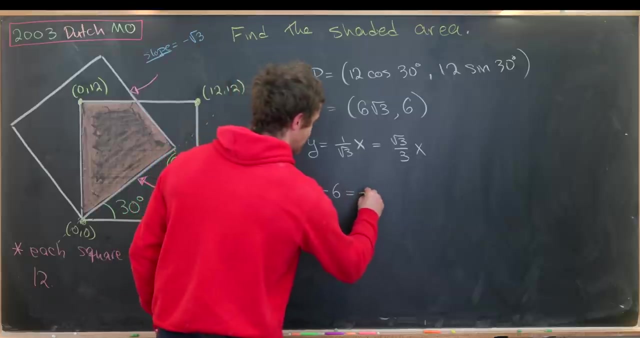 So the slope here will be negative, square root of 3.. And now we can use point slope form to find the equation of that line, So that'll be y minus the y-coordinate of a point, So that'll be 6.. We can use that point right there. equals slope. 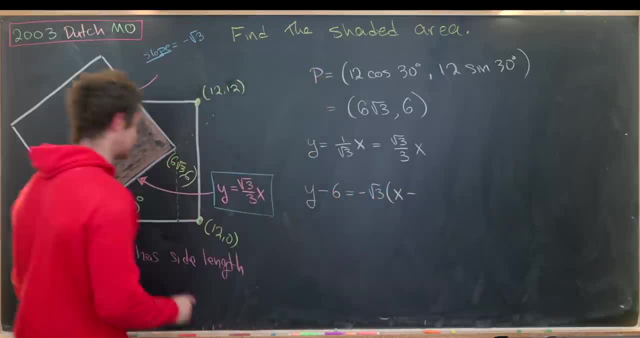 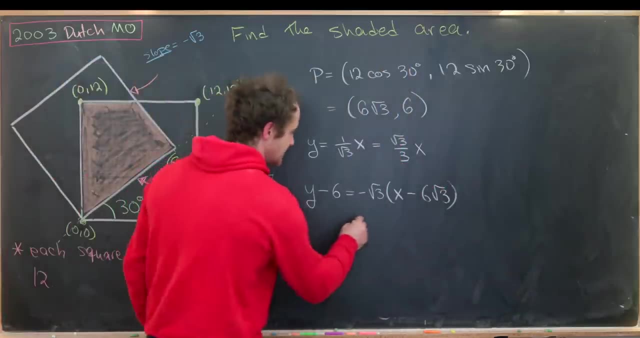 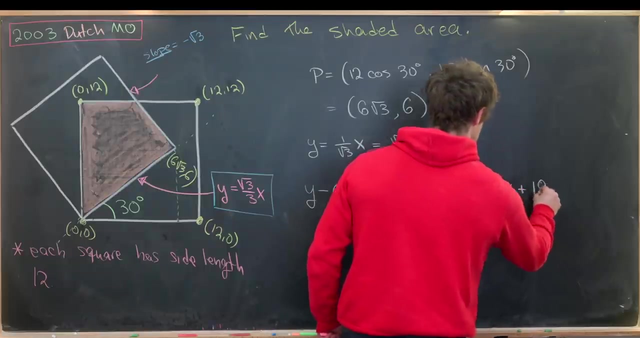 So that's negative square root of 3 x minus the x-coordinate of the point. So that'll be 6 times the square root of 3.. So let's see what that gives us. We'll have negative root 3 plus times x plus. I think that's going to be 18.. 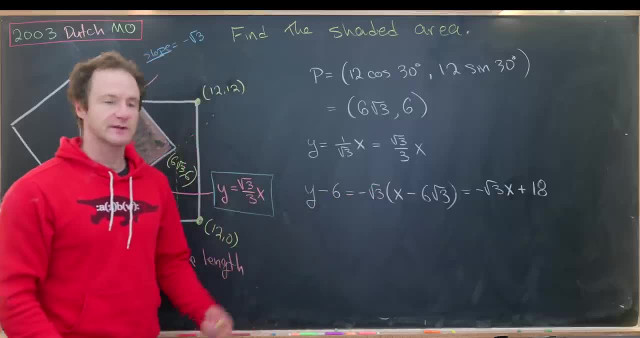 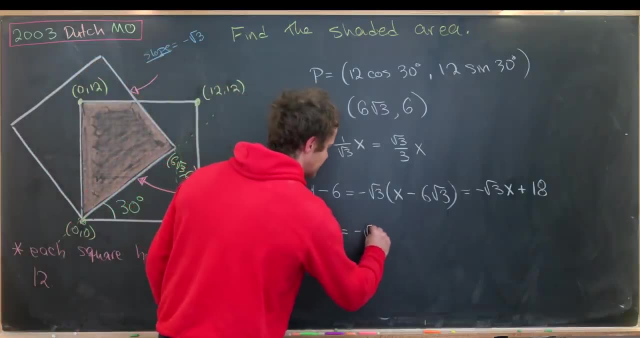 So we get that from root 3 times root. 3 is 3 times 6 is 18.. And then the minus signs cancel. So in the end we see that y is equal to negative square root of 3, x plus 24.. 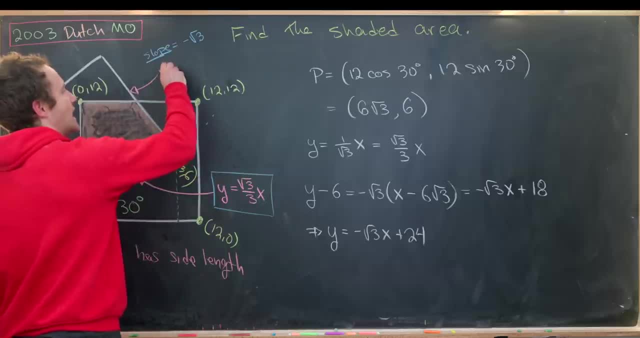 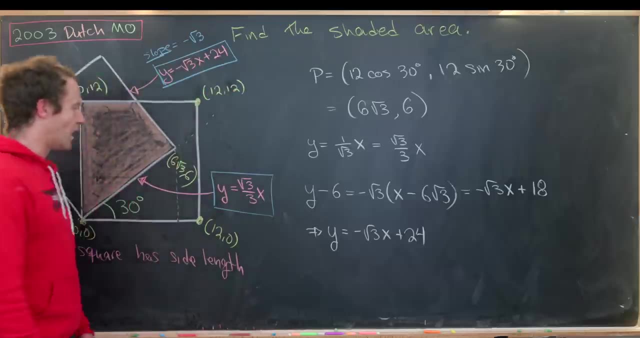 Okay, so let's include that here We have: y equals negative root, 3 x plus 24.. And we have one last thing to calculate, And that's the coordinate of this point right here. So maybe I'll call this point q for the time being. 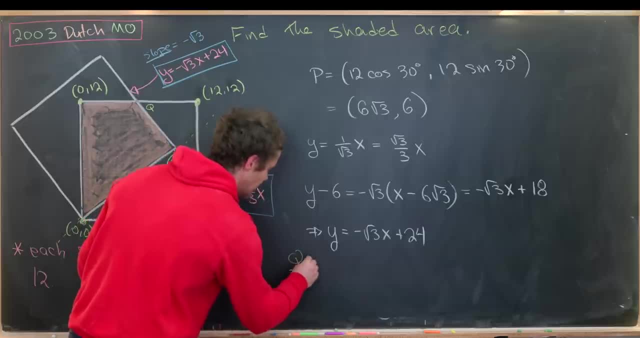 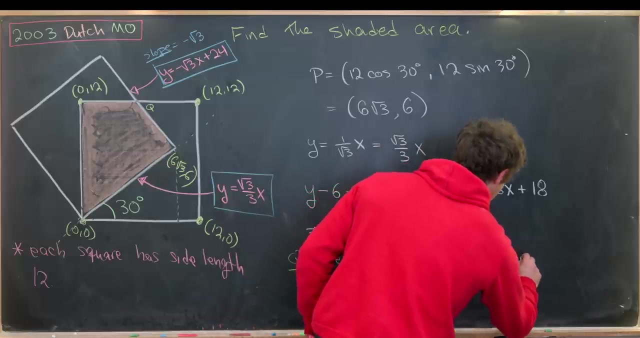 And then we'll calculate it over. So I'll write q and we'll calculate it. given the fact that it's the intersection, So I'll write it like this: The intersection of our line y equals negative root, 3 x plus 24, and the line y equals 12.. 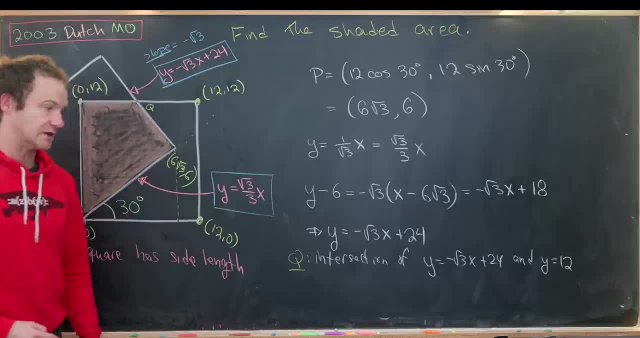 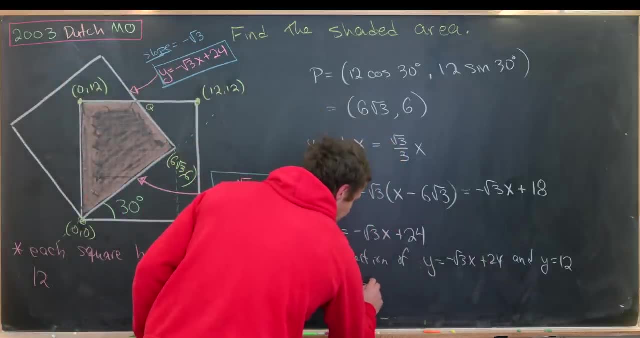 Notice this horizontal line up here has equation y equals 12.. So that'll be pretty easy to calculate. We'll just set y equal to 12 over here And we'll end up with negative root. 3 x plus 24 equals 12.. 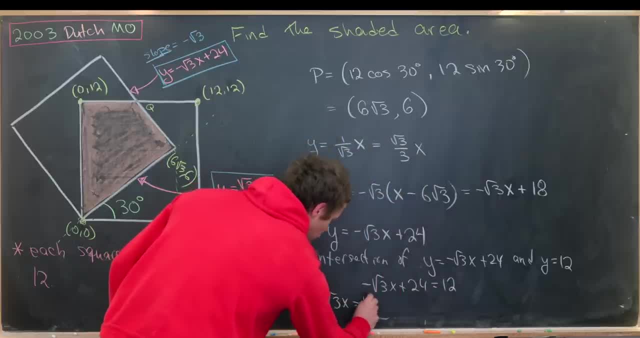 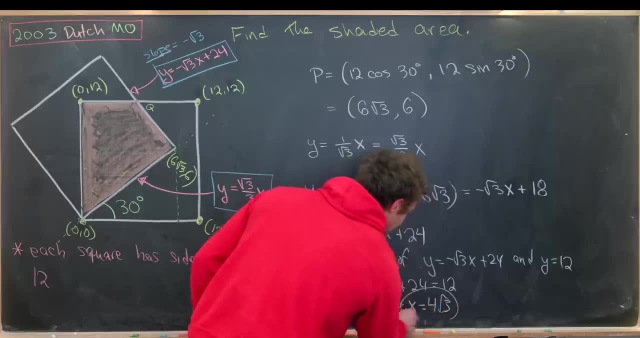 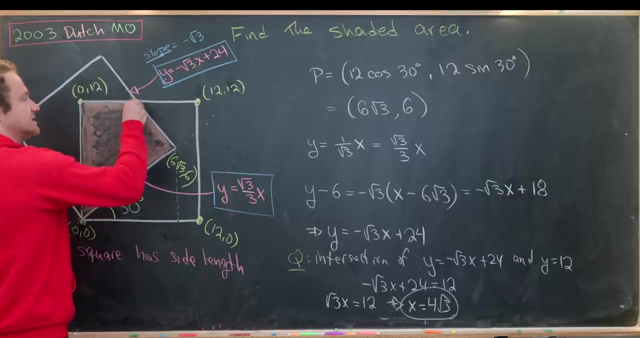 Which means root 3 x equals 12.. But in the end that tells us that x is equal to 4 times the square root of 3, after a little bit of arithmetic. Okay. so now I'll erase this q, since we know what it is. 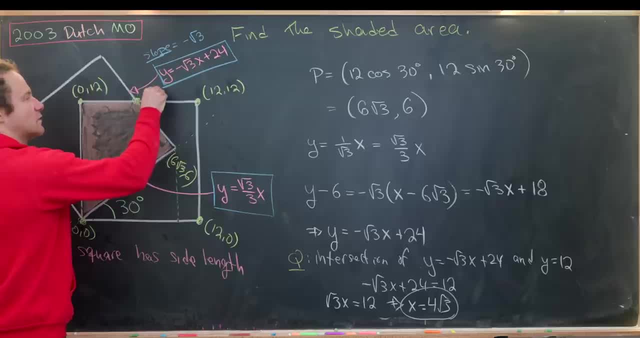 And let's include this point right here. So the x coordinate is 4 root 3.. And in the y coordinate we have 4 root 3.. And the y coordinate is obviously 12 because it's along that horizontal line which is based at y equals 12.. 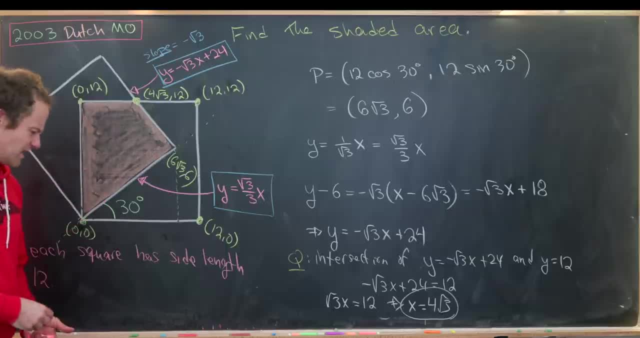 Okay, so now we have all of these parts. Maybe, before we erase things and start calculating, let's give names to some of these things. Let's maybe call this thing down here l1.. And we'll call this thing up here l2.. Okay, so now let's erase this calculation and we'll do our final area calculation. 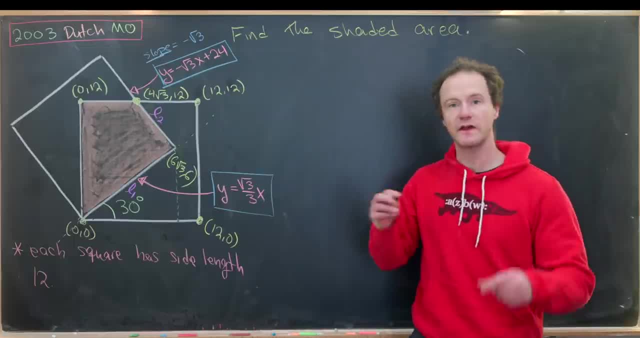 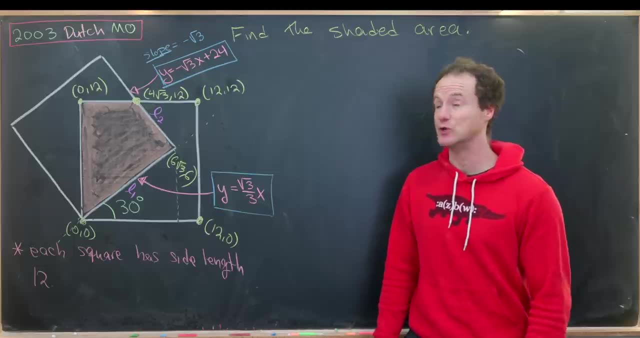 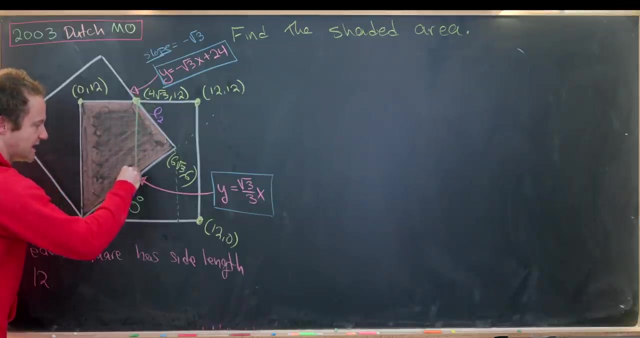 Okay, so now that we've got all of these parts calculated, we're ready to finish it off. Like I said, the way we're going to do it is quite ridiculous, And we're going to do it by taking two integrals, So we can split this up into two parts. we can drop a vertical line from this point right here. 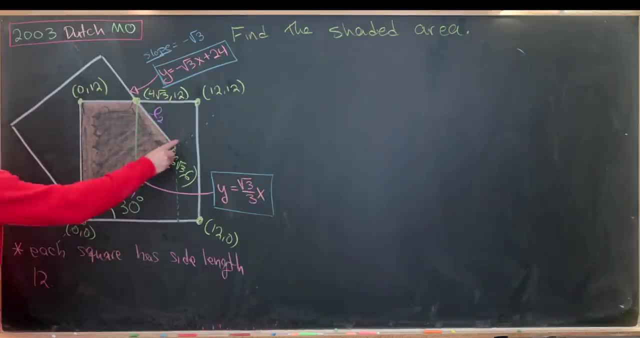 to wherever this vertical line intersects, this line. It doesn't really matter. We know the x coordinate is 4, root 3, and that's all we really need, And then we could name each of these Areas. maybe we could name this area a1 and this area a2.. 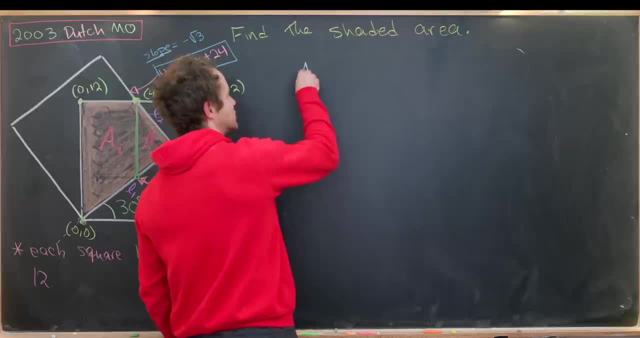 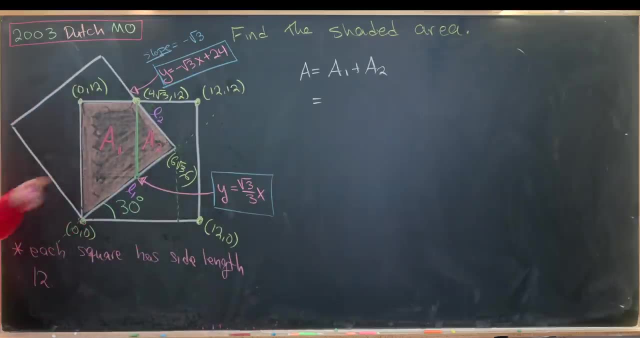 And then let's notice that our goal area, which I'll just call a, is a1 plus a2.. But now a1 can be rewritten as the integral of this vertical line equation minus l1's equation. This vertical line equation is 12 and l1's equation is that. 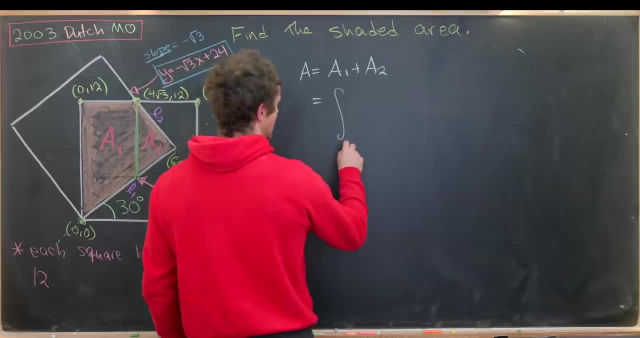 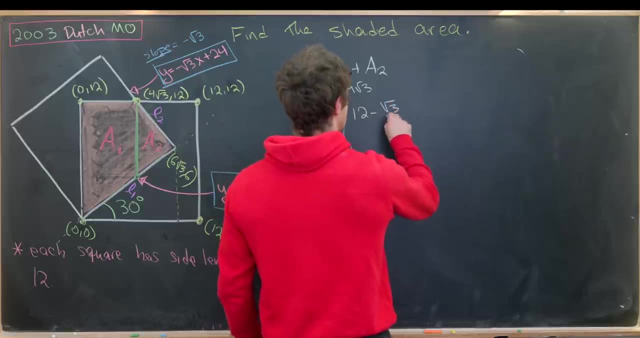 Over there. so we have something like this: This is going to be the integral from 0 to 4, root 3 of 12 minus root 3 over 3 times x dx. Again, we've got our top curve minus our bottom curve. 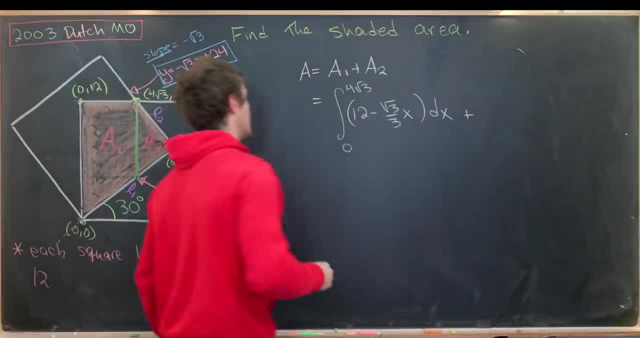 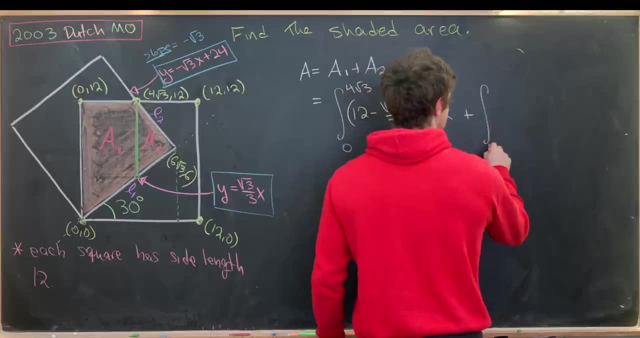 Okay, nice, and now we'll add that to the area 2.. But in this case l2 is our top curve and l1 is our bottom curve. So we have the integral from 4 root 3 to 12.. to 6 root 3 of. so our top curve is that. so that's minus root 3x plus 24, minus the bottom curve, which. 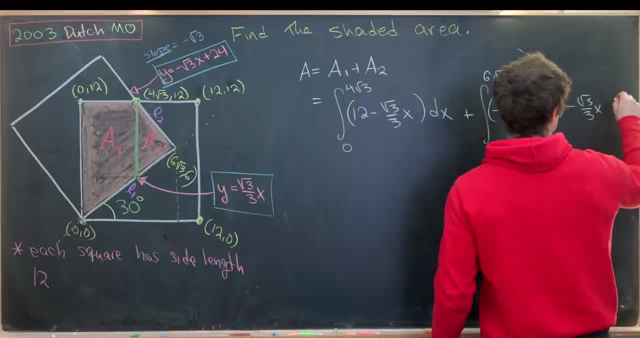 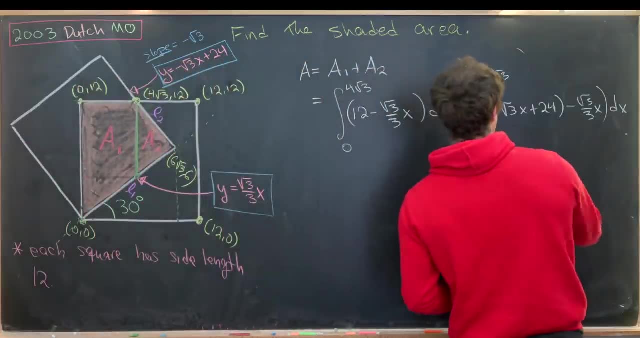 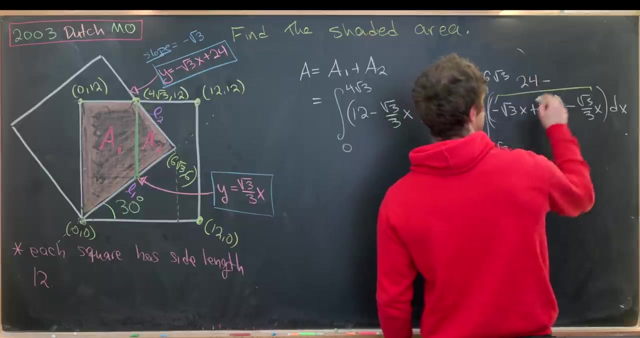 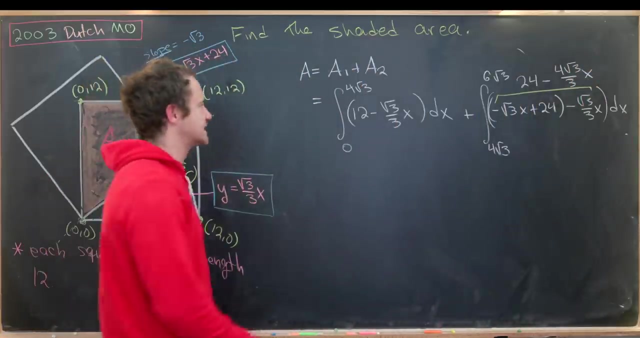 is root 3 over 3 times x and then dx around the whole thing. but maybe we should do a little bit of calculation here before we get going. notice this can simplify to 24 minus. let's see that'll be 4 root 3 over 3 times x when everything is said and done. so now let's get to the final. 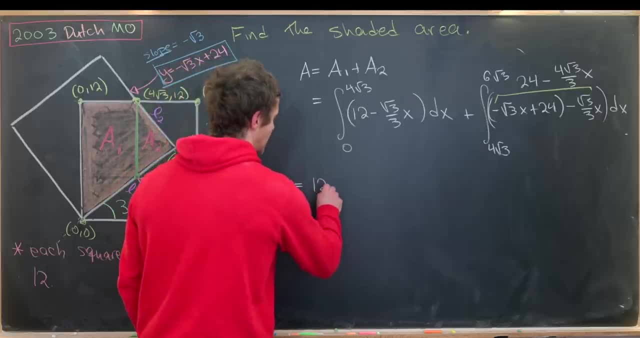 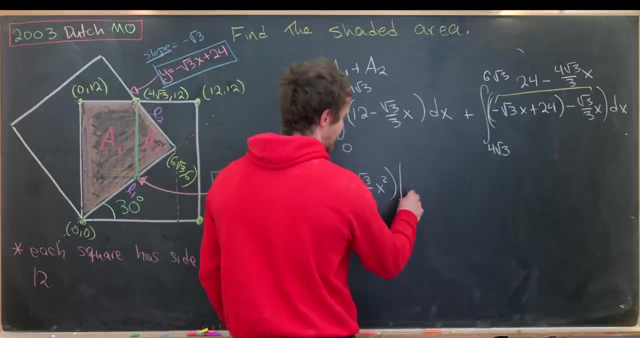 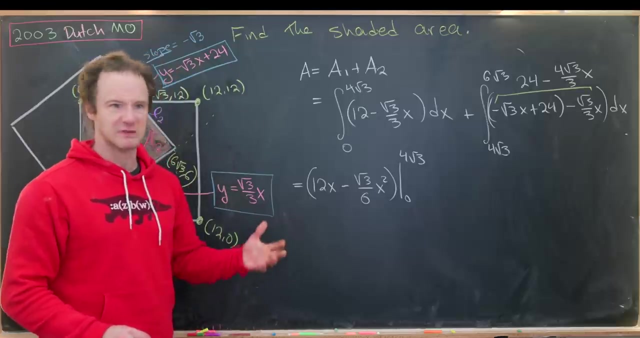 calculation. so this is going to give us 12x minus the square root of 3 over 6 times x squared. we need to evaluate that from 0 to 4 times the square root of 3 over 6 times x squared. so there, I just took the antiderivative and plugged in the endpoints. that's not too bad, then we've got. 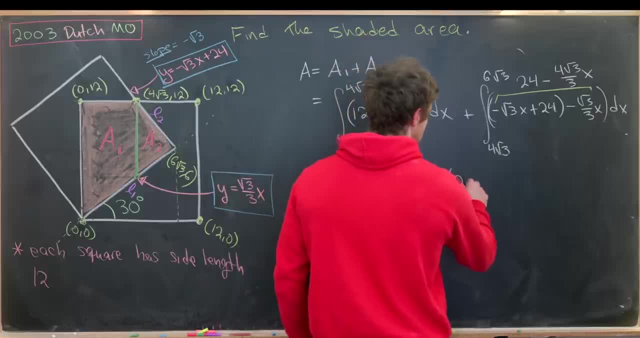 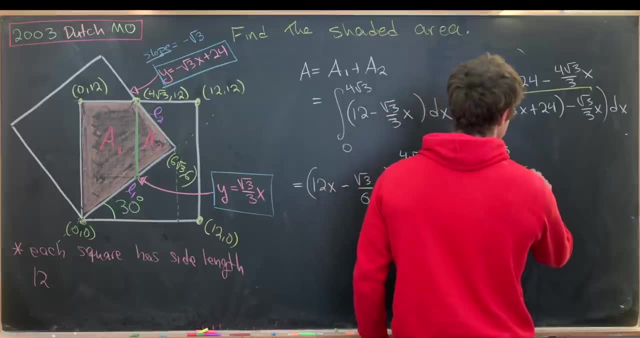 something similar over here. so let's see, that'll be plus 24 times x minus. that'll be 2 times the square root of 3 over 3 times x squared again. we need to evaluate it on those endpoints though, so that's 4 root 3 and 6 root 3, so we've got something like that cooking up so far. 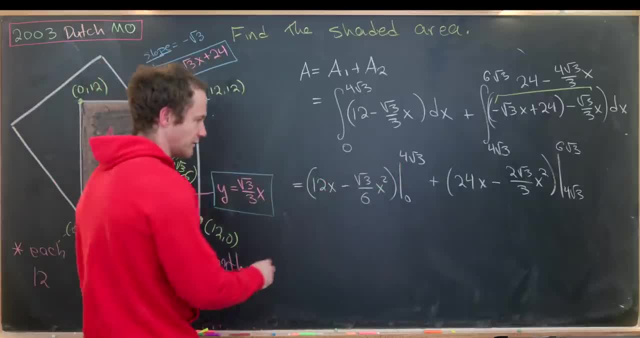 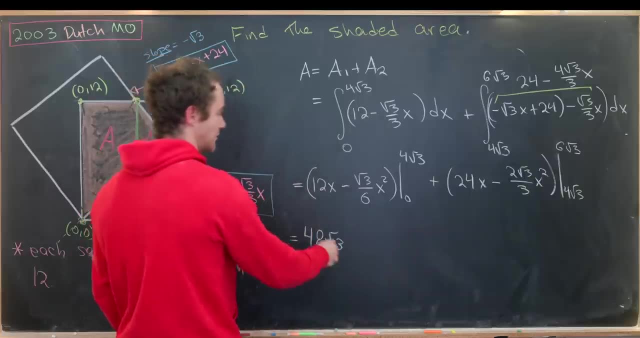 okay. so now we're going to do a little bit of calculation here. so we're going to do a little okay. so let's notice, when we plug in 4 root 3, we'll have the following simplification: this will give us 48 times the square root of 3 from this term minus. well, let's see if we square this we. 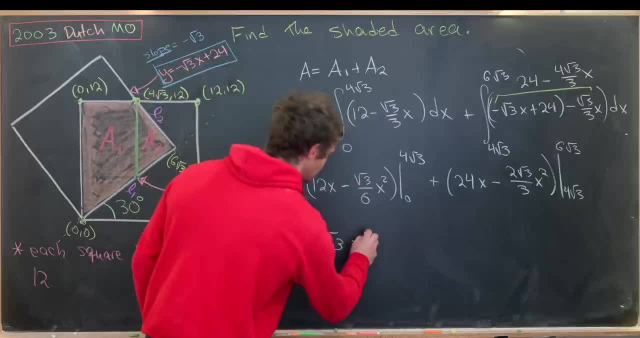 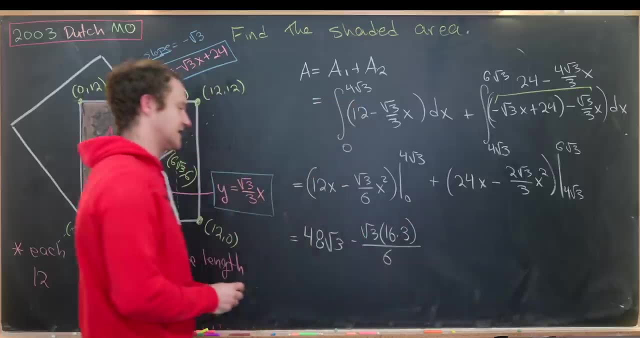 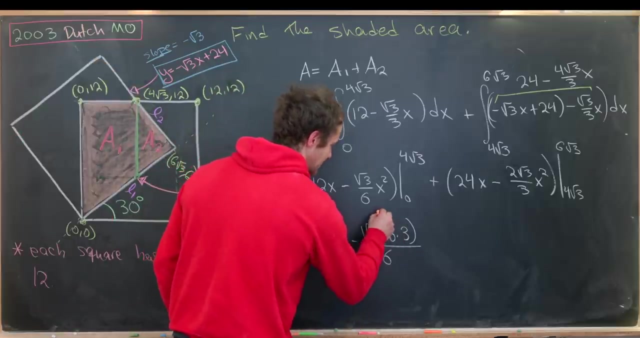 get 16 times 3. so let's write this out so we know exactly where it's coming from. so we have the square root of 3, 16 times 3 over 6. now let's simplify. so notice this 16 can be rewritten, as I think maybe it's best to rewrite it as 8 times 2, and then this 2 and this 3 can cancel this. 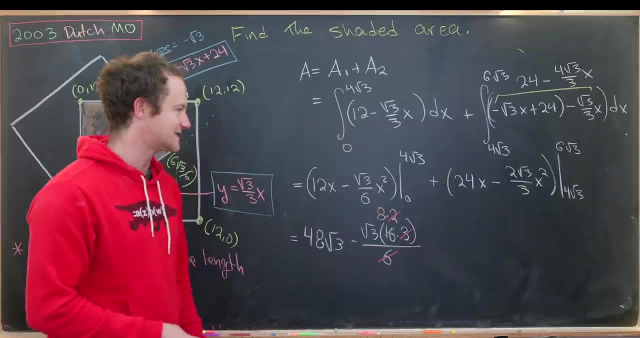 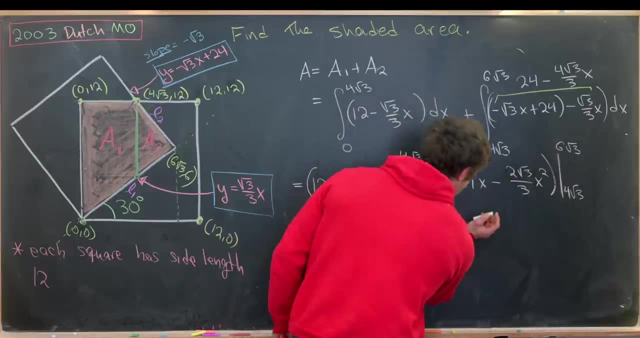 6, so we're left with something like that. okay, now we'll have something similar over here. so this will be plus 24 times 6 root 3, minus 4 root 3, so that'll give us 2 root 3 multiplied by 24. we have.